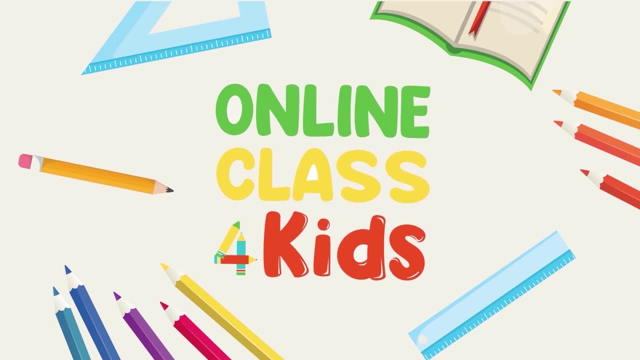 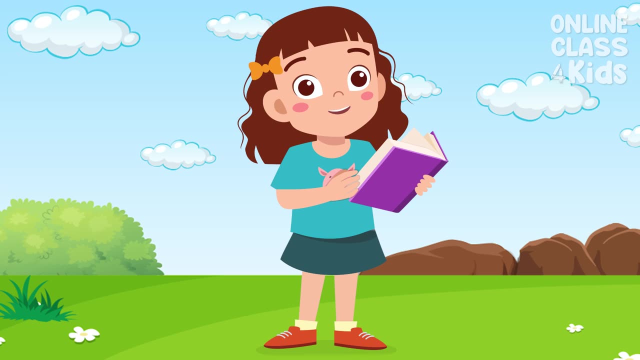 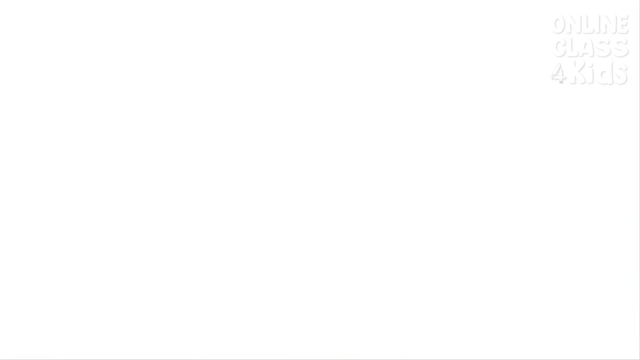 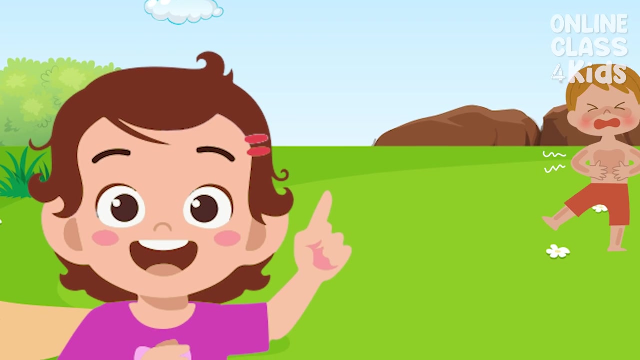 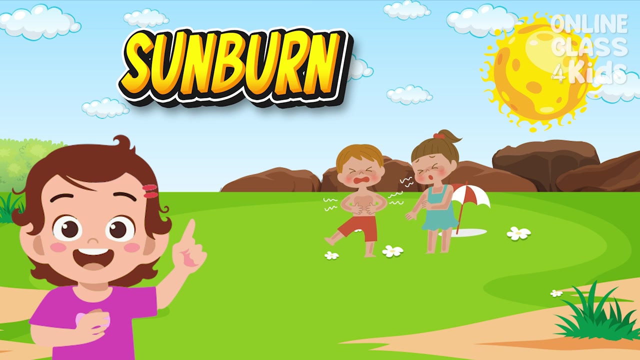 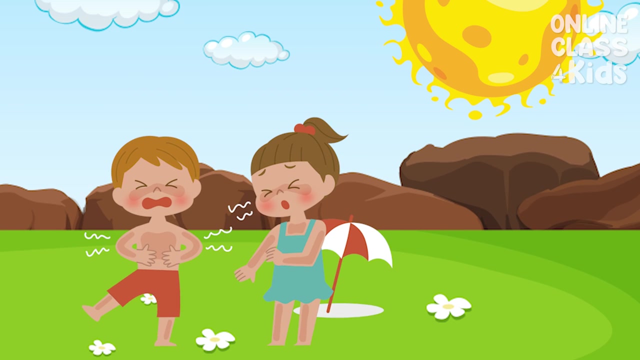 Online Class for Kids. Hello there, Welcome to another exciting episode here at Online Class for Kids. It's so fun to play outside, But do you know what happens after playing under the sun for a long time? That's right, You will get a sunburn. You don't want that, don't you? 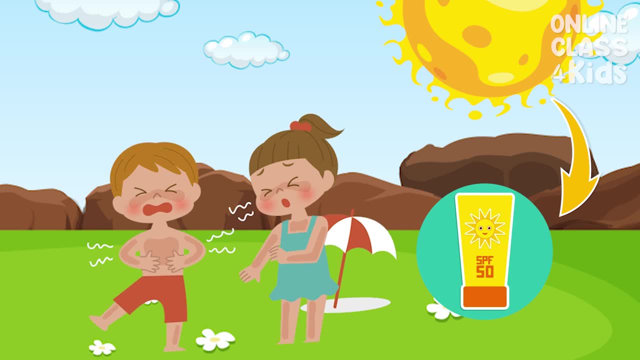 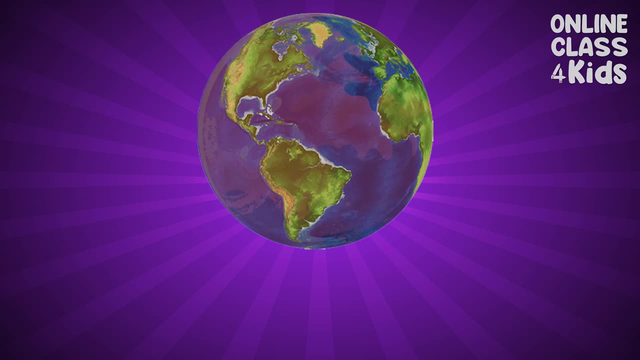 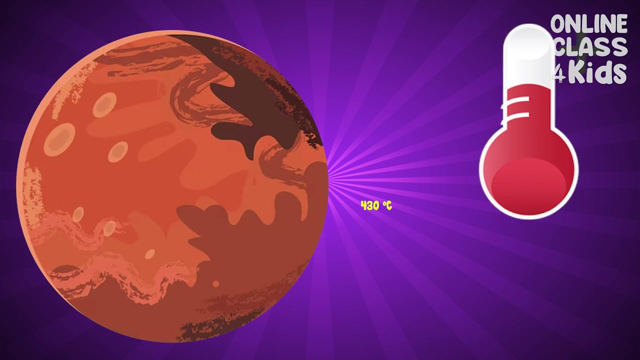 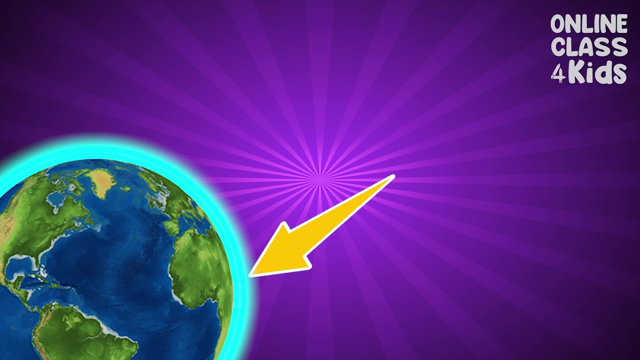 We can protect our skin by wearing a sunblock. If the Earth had no protection of some sorts, our planet would end up like Mercury, Where it can get super hot, up to 50 degrees, 430 degrees Celsius. This protection is otherwise known as the atmosphere. 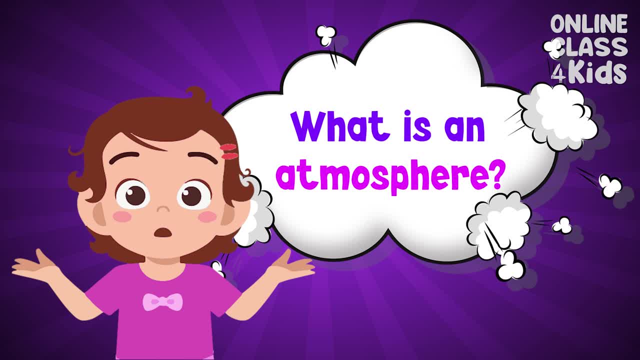 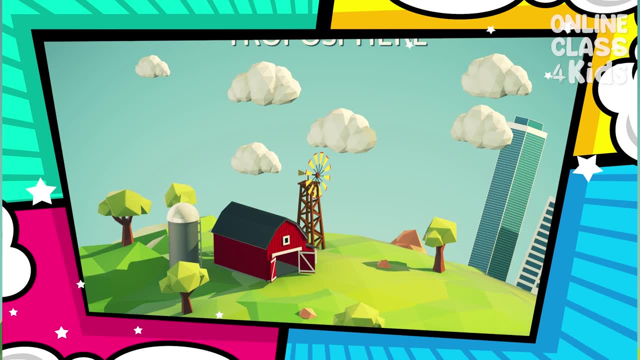 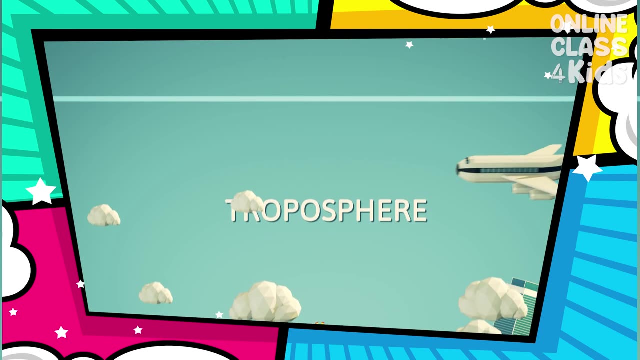 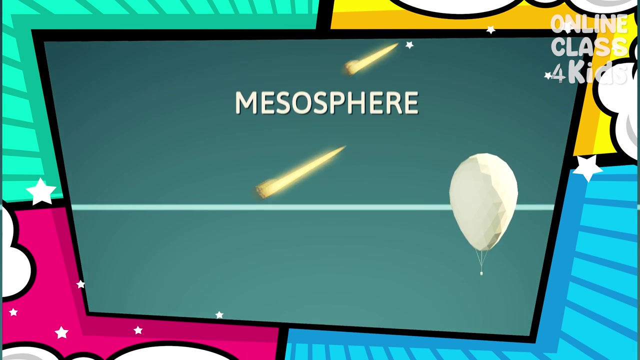 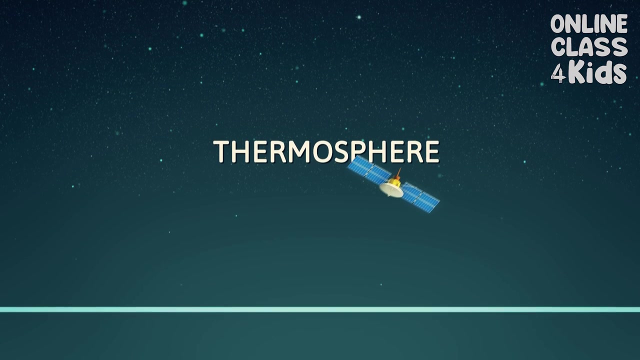 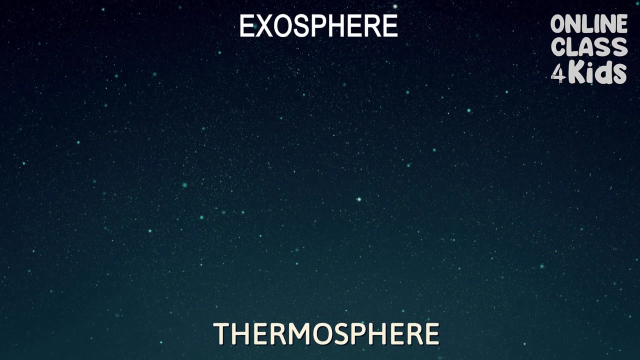 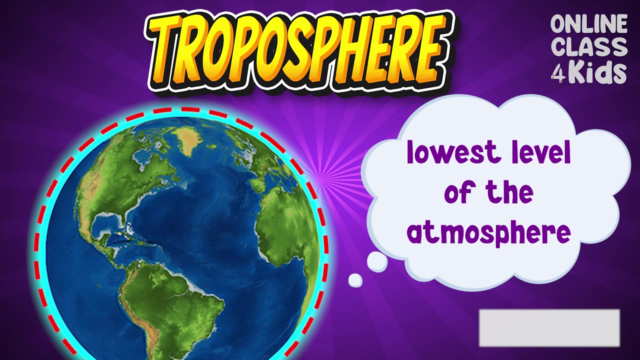 What is an atmosphere? Let's learn more about it. The Earth's atmosphere is divided into five layers: The troposphere, Stratosphere, Mesosphere, Thermosphere And exosphere. The troposphere: It's the lowest level of the atmosphere. 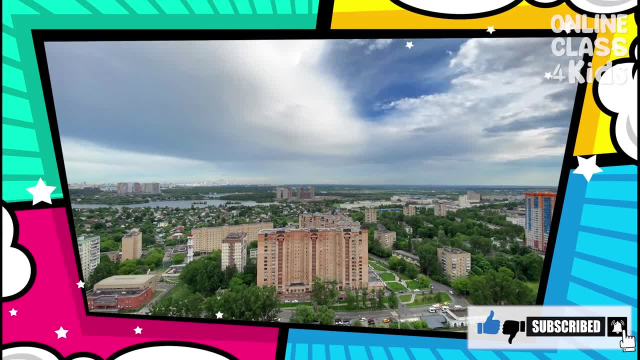 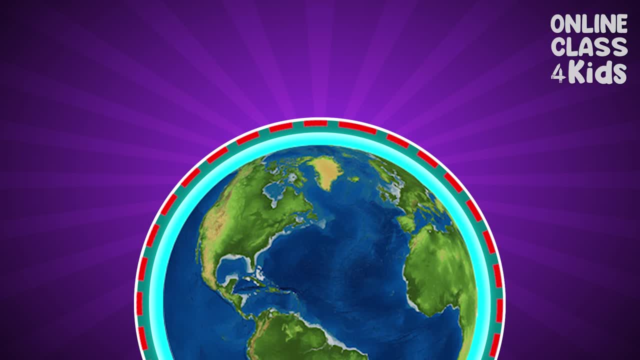 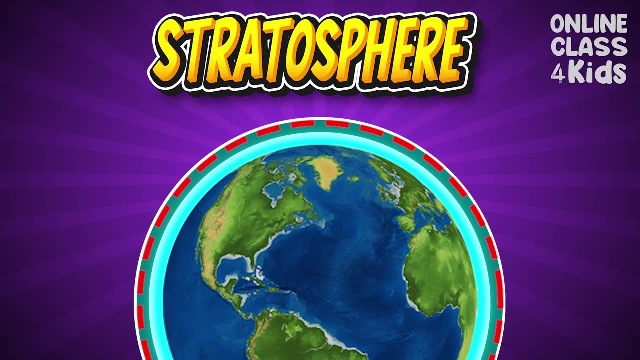 It is where we live. It is where the different weather takes place. The next layer is the stratosphere. This is where you find the ozone layer. The ozone layer protects us from the sun's harmful UV rays. The ozone layer protects us from the sun's harmful UV rays. 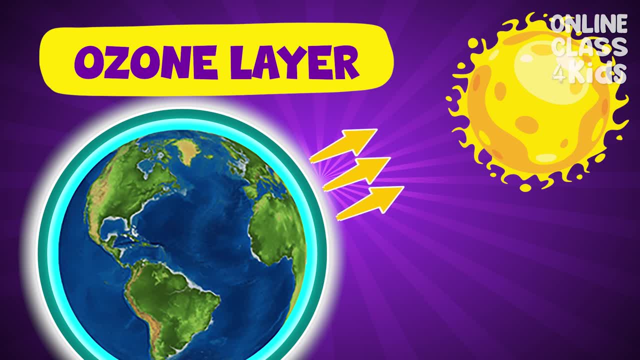 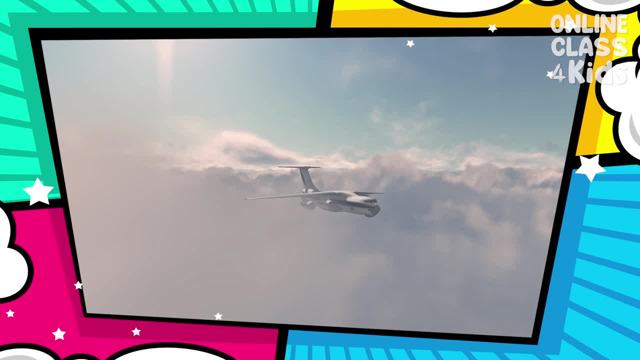 The ozone layer protects us from the sun's harmful UV rays. The stratosphere is also the highest layer that jet planes can reach. The stratosphere is also the highest layer that jet planes can reach. The stratosphere is also the highest layer that jet planes can reach. 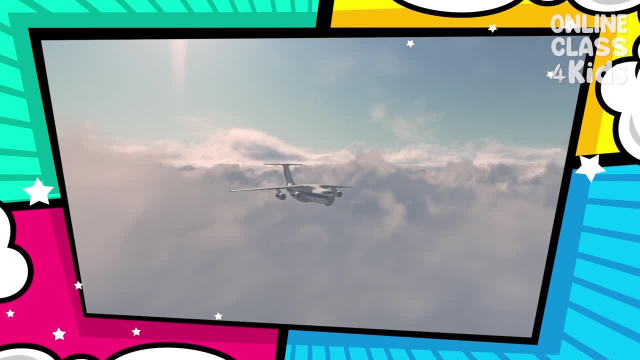 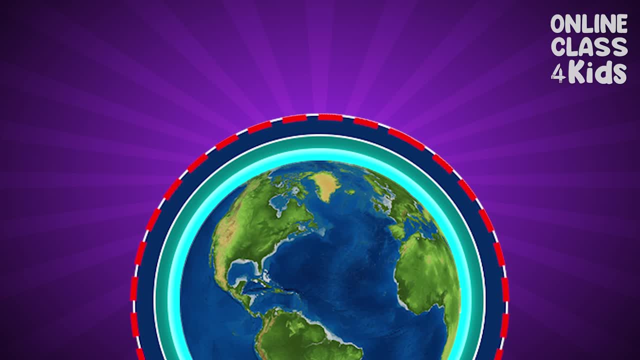 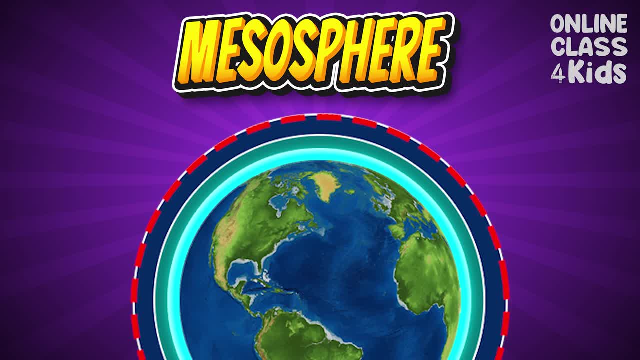 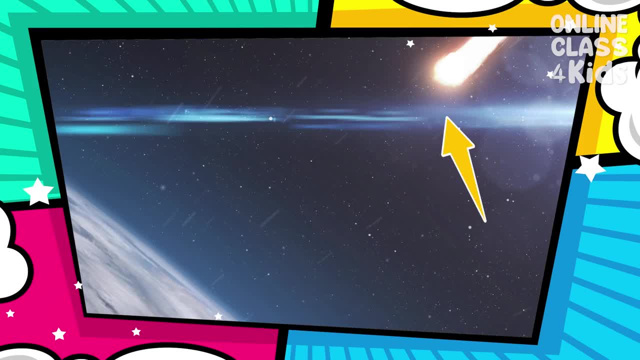 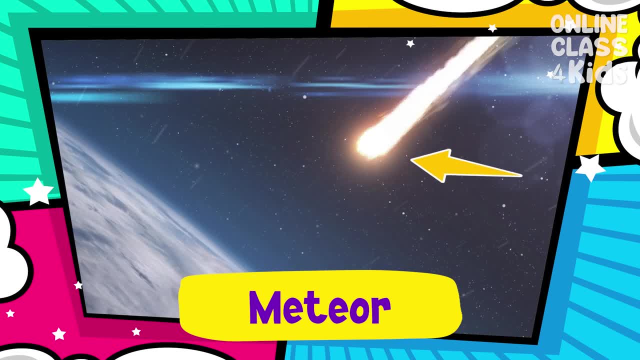 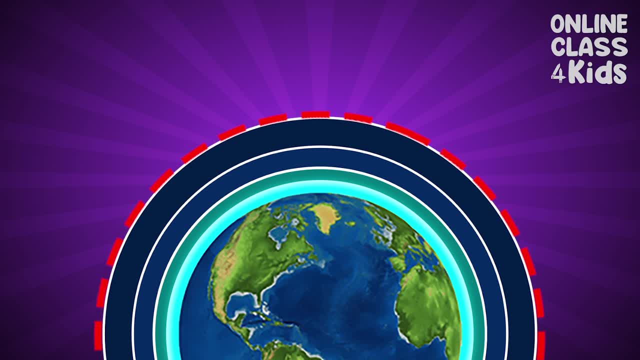 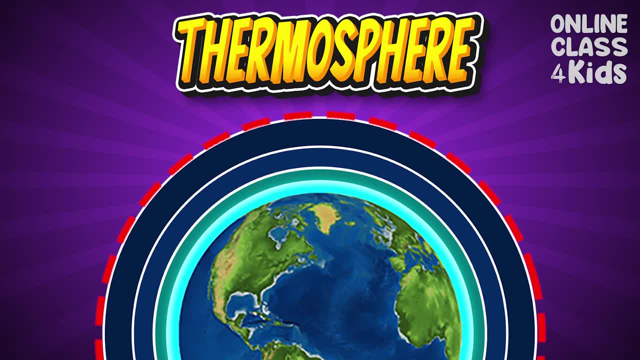 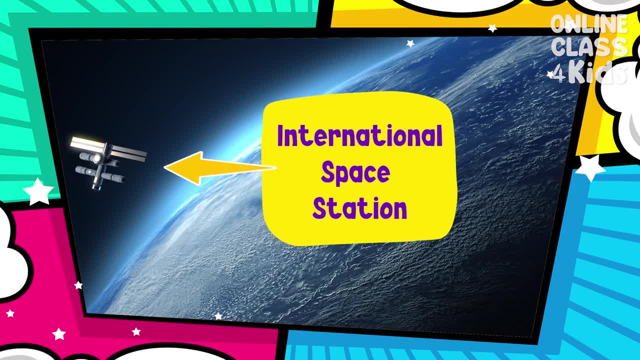 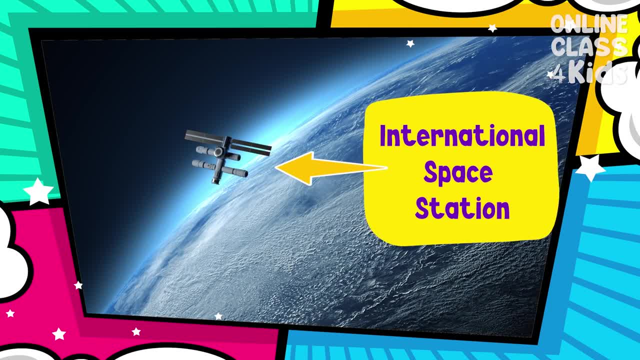 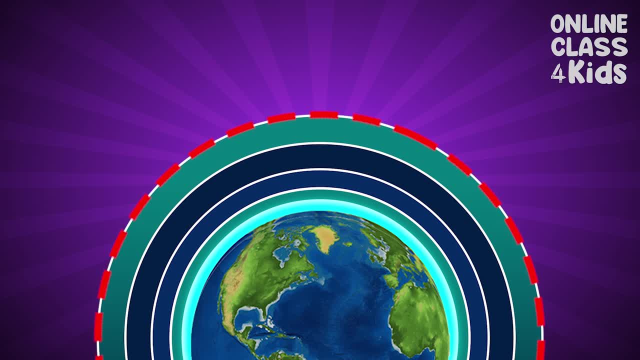 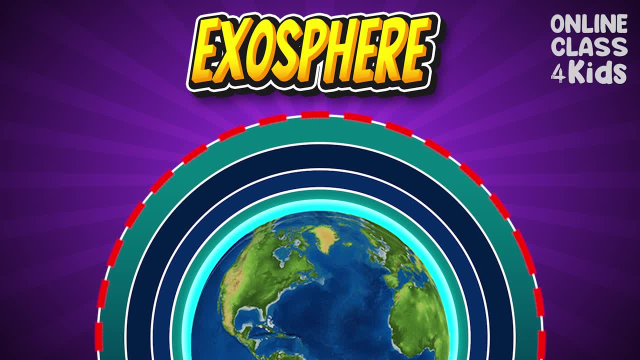 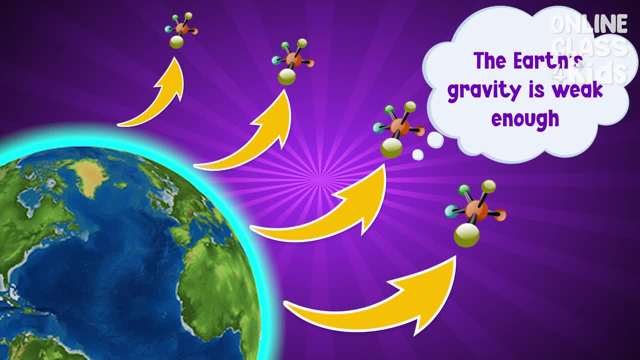 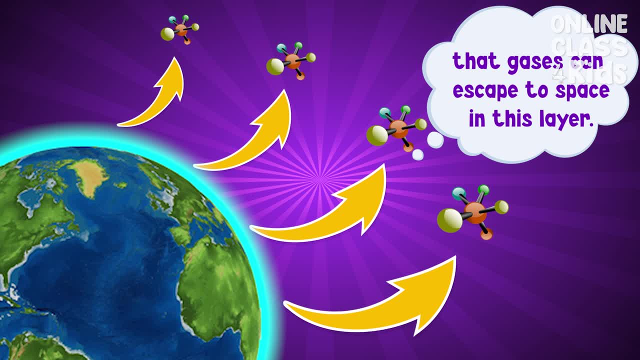 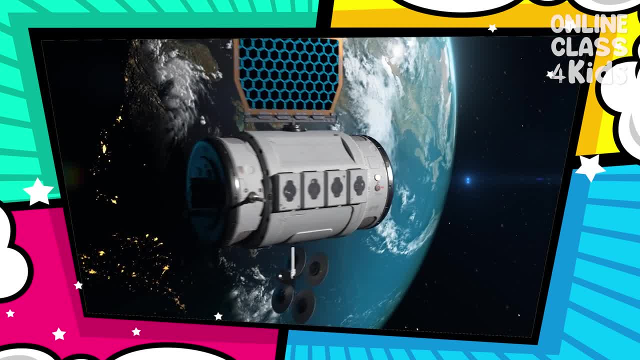 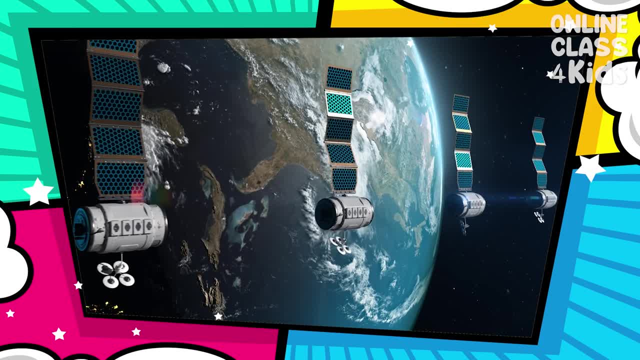 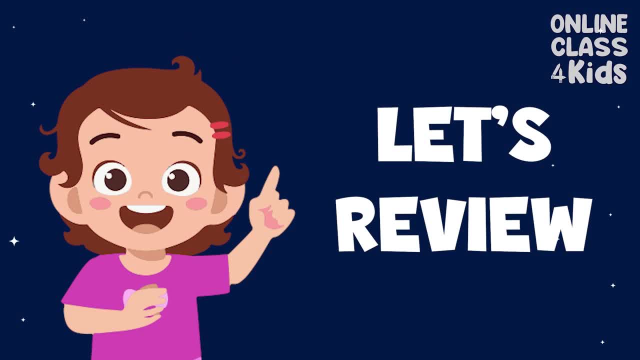 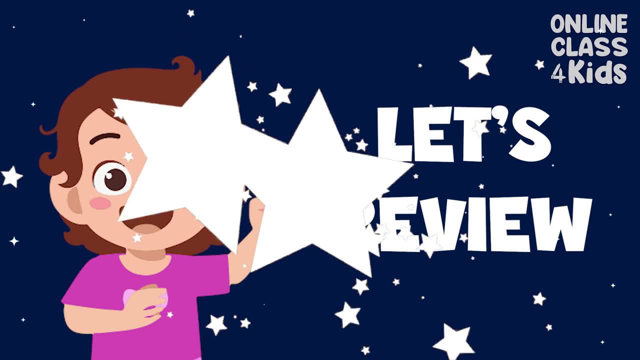